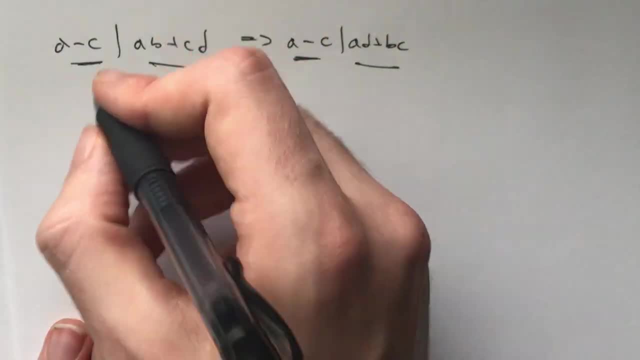 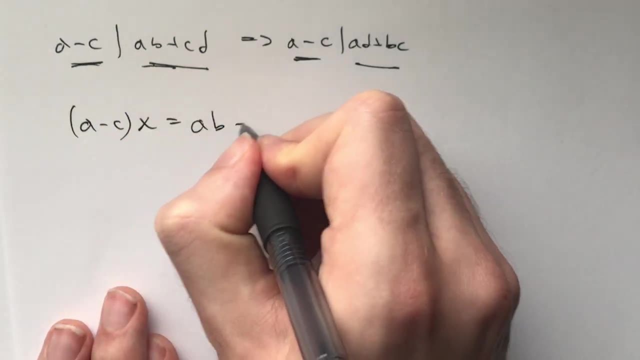 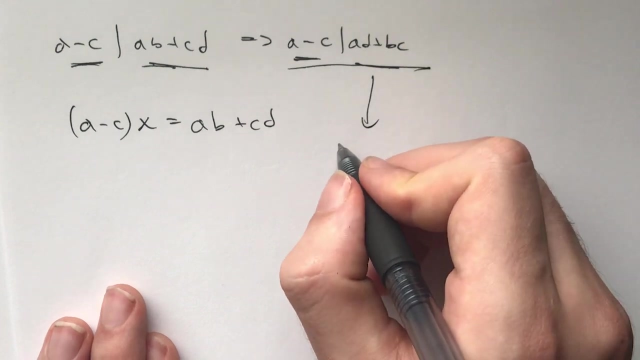 I'm trying to like teach you some lessons in number theory now through problems. So if this divides this, that means there exists an integer x, such that a minus c times x is a b plus c, d. Great. What does it mean for a minus c to divide this? Well, it would mean that there exists an. 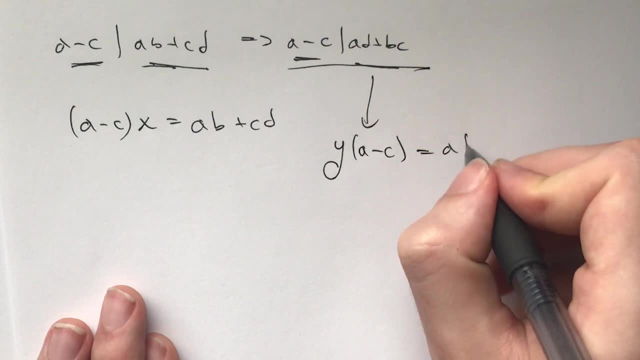 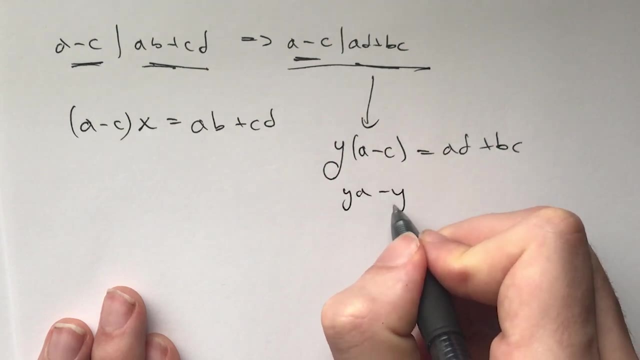 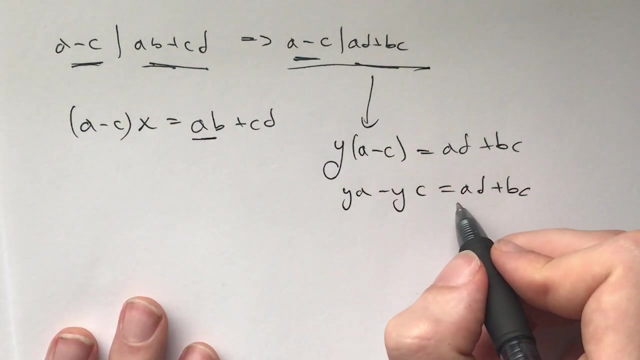 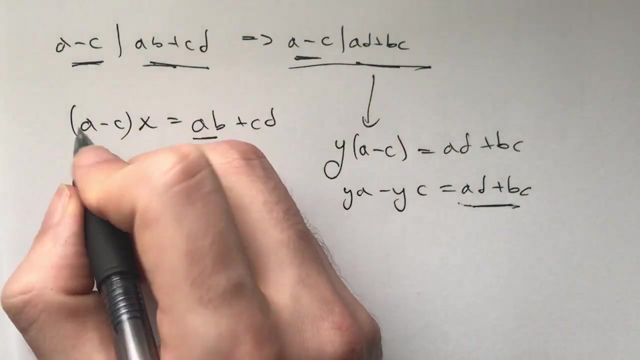 integer y such that y times a minus c is a d plus b. Great, So now this is: y a minus y c is a d plus b c. Now, how can we transform these things here into these things here? That is basically what our question is. So what can we do? 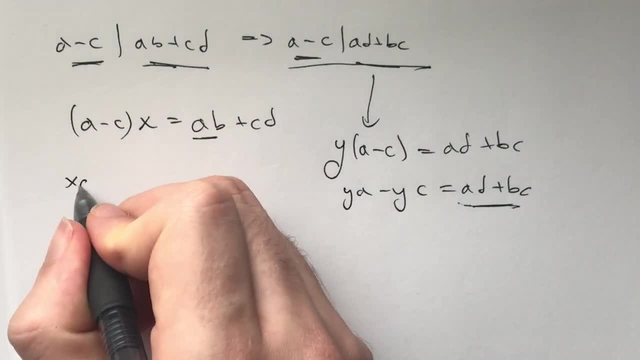 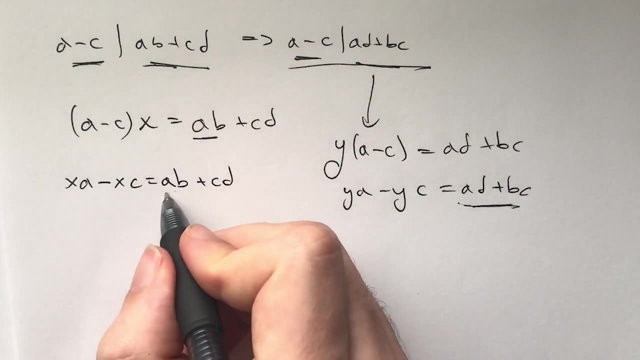 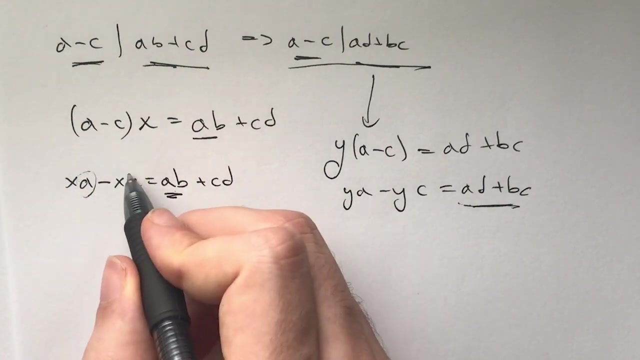 And this is one way of thinking about this. Well, this is x a minus x c, is a b plus c d. Can we get rid of a b somehow? What if we add or subtract something to maybe have a minus c on this side? 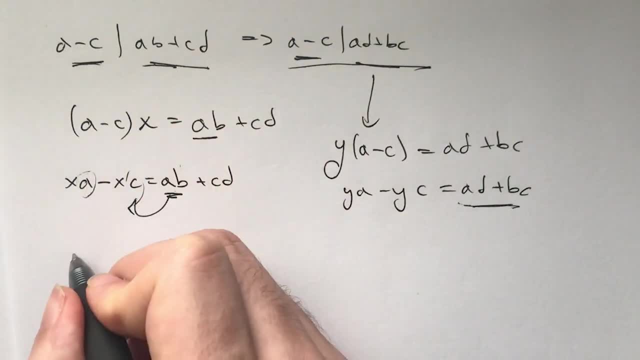 Then we can move it here. Actually, you know what? Let's move a- b here. Then we have x a minus x c, minus a b plus c d. Okay, Now how do I create a minus c? Well, it's going to be minus a b. 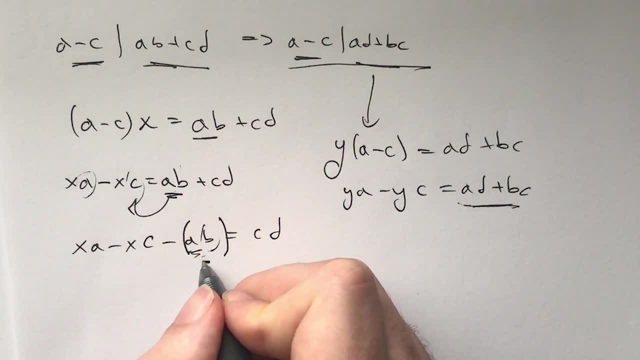 and I'm going to need to get b out, right? So I need to add minus b c, The minus minus. I need to add plus b c here, right? So all I get I'll get x times a minus c, minus b times a minus c, c, d, plus. 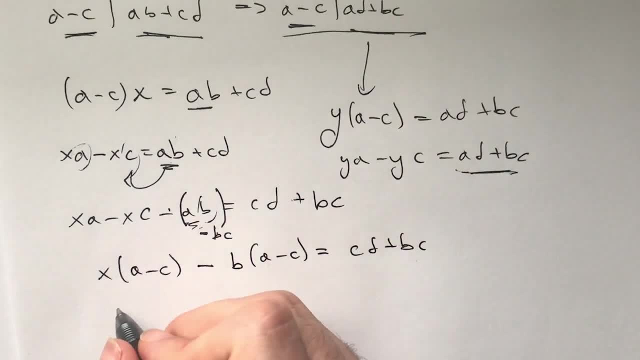 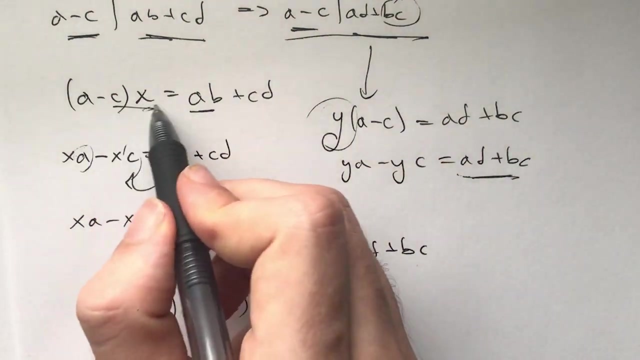 b c right. So now, from here, I get that x minus b times a minus c is equal to c d plus b c. And now, look, I've gotten the one of the things I need, and I may be able to now get y. You know, from here, from this x I'll need. 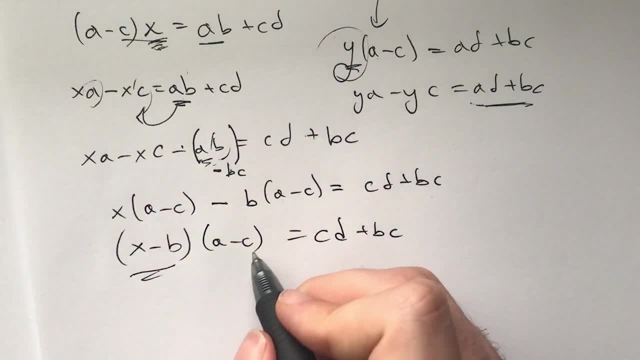 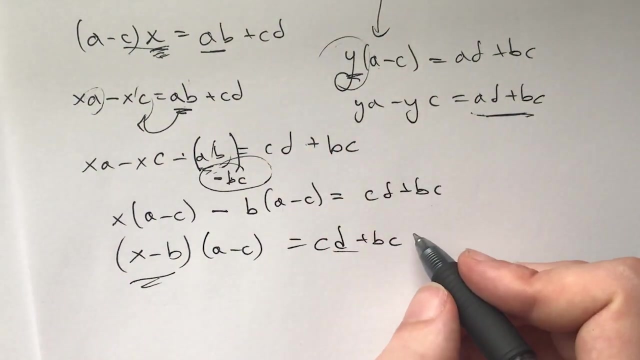 to create a y. And now, what did I do? I subtracted. So what I actually did here was: I added. so what did I add? I added b c to both sides. So let me add now what do I need? b c. let me add a d to both sides. 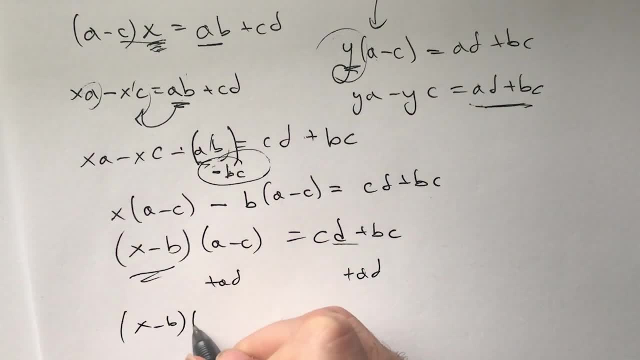 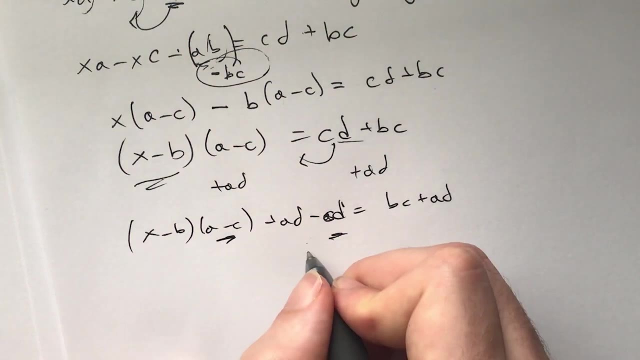 a d and a d. I have x minus b, a minus c plus a d. Let's move this to the other side. Then we have a d minus c. d is b, c plus a d. And now again I can factor this out: the d out, the d out, and I'll get d times a minus c here. 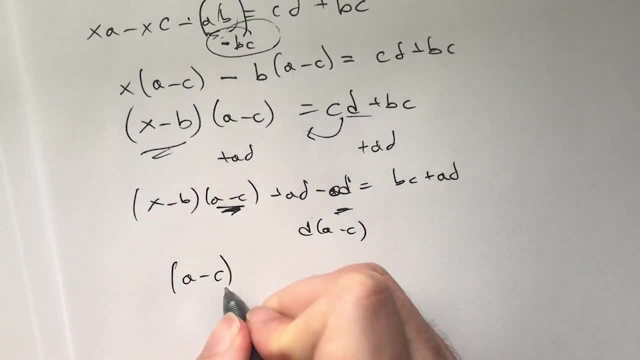 a minus c. I factor those out and I get a minus c times. x minus b minus d is b c plus a d. Now for y equals this: It's minus b minus d. We have y times a minus c is b c plus a d, which implies that a minus c divides b c plus a d. 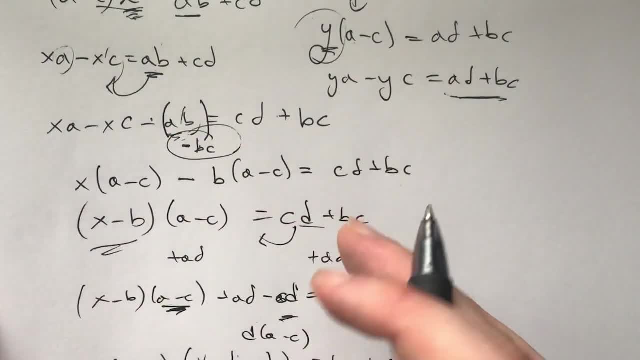 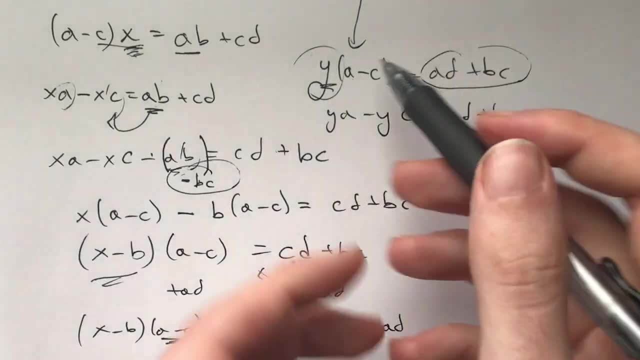 And now this is one method that you can use. There's not really there's not any big of a structure, it's just like I need to have this on this side. so I add it: I need to get rid of these on these sides, and the only way I can get rid of it. 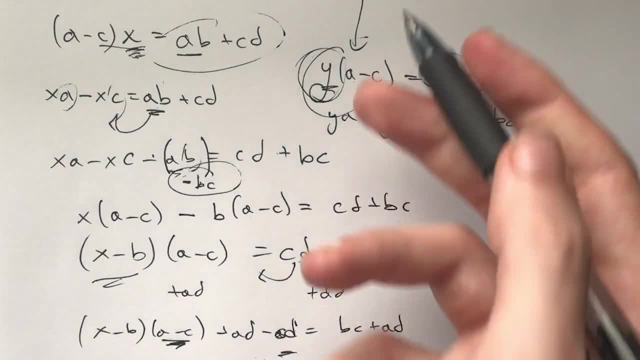 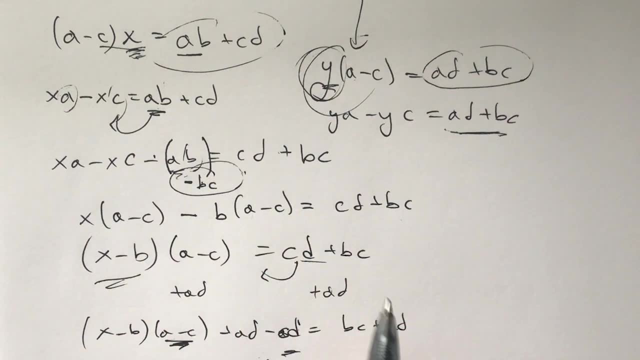 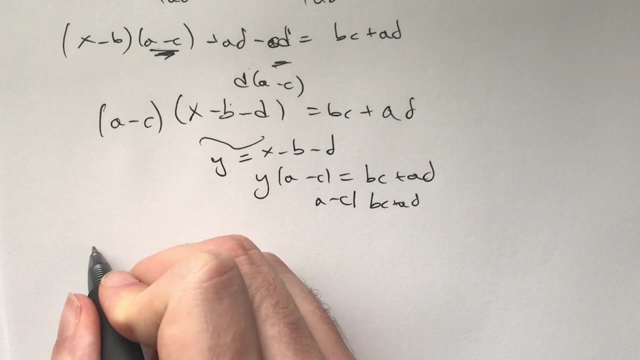 is to incorporate it into this. y times a minus c, And to do that, I move it on the other side. What I need to incorporate into a minus c, well, i need to add the thing i need to add to get this, and. but there's a different way of solving this as well, and this is also looking at something else. it's 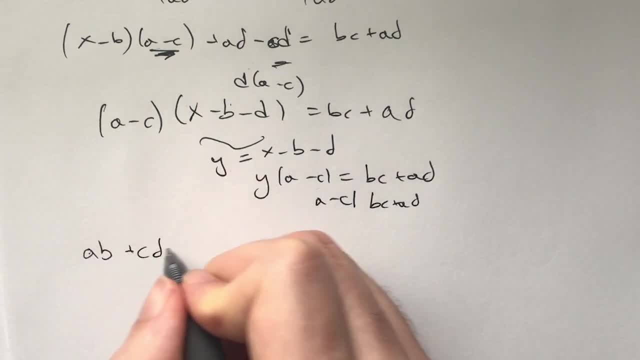 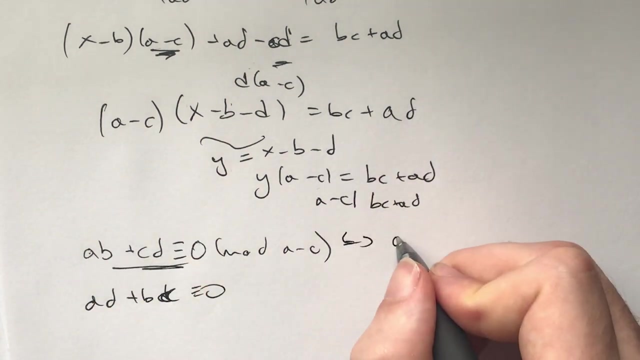 looking at modular arithmetic. so a b plus c, d is congruent to zero modulo a minus c, correct? and we need to prove that a d plus b, d, b, c is also zero. right now, this is equivalent to a b is congruent to negative c d modulo a minus c. and now i invite you to pause for two to five minutes and see if 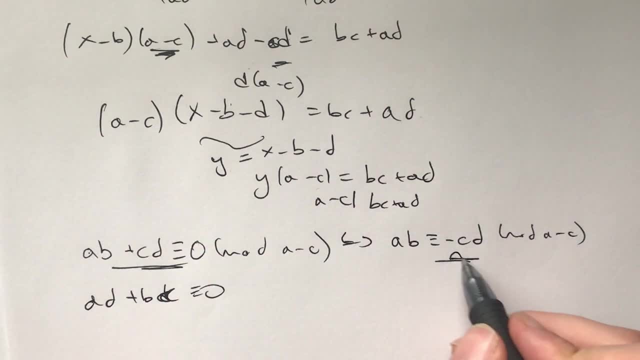 there's anything you can do with this. well, the question is, how can i change this into something else? what is a b also congruence to modulo a minus c? well, a b is congruence to c b, right modulo a minus c. and how is it that i know this? actually, is it? yeah? 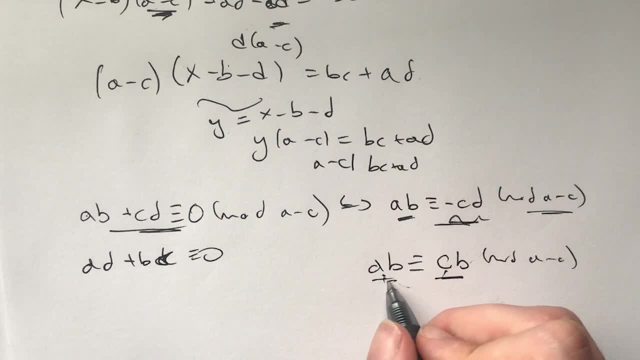 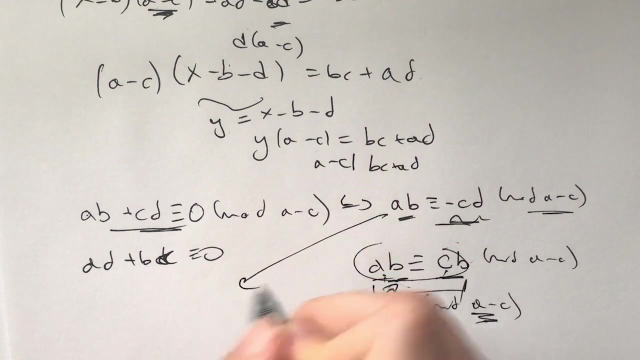 that. why is it? why is this true? well, this is true if, and only if, is congruent to c modulo a minus c. and now this is true because a minus c divides a minus c, and it's like you can work with modular arithmetic by multiplying stuff together to get new things. and now this means that